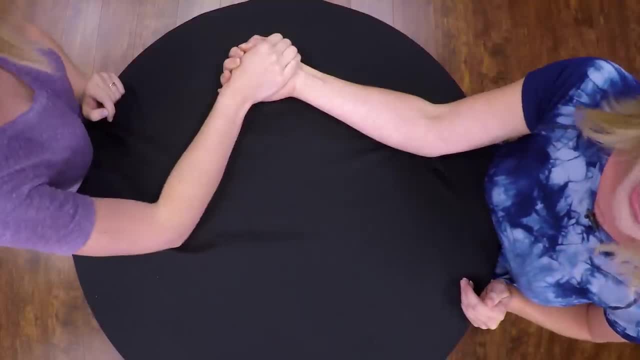 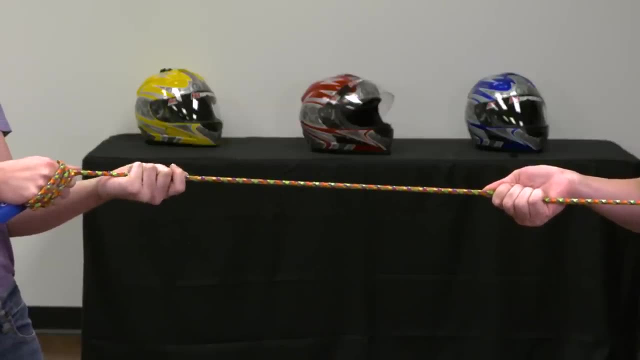 object accelerates in the direction of the net force and Summer wins Same in a tug of war. If both sides are pulling with equal force, there's no movement. That's balanced. But if one side pulls harder, it's unbalanced, which means there's a greater force on one. 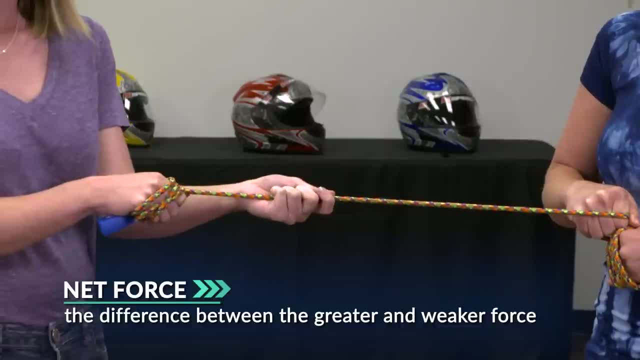 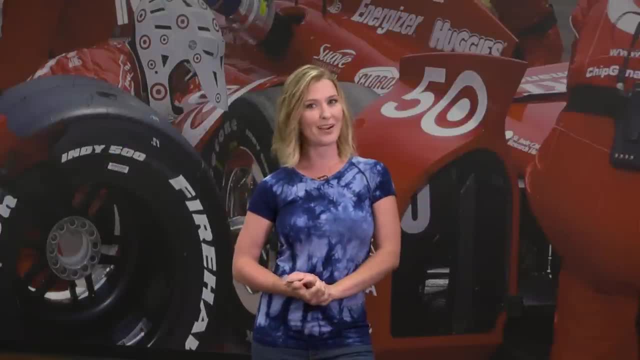 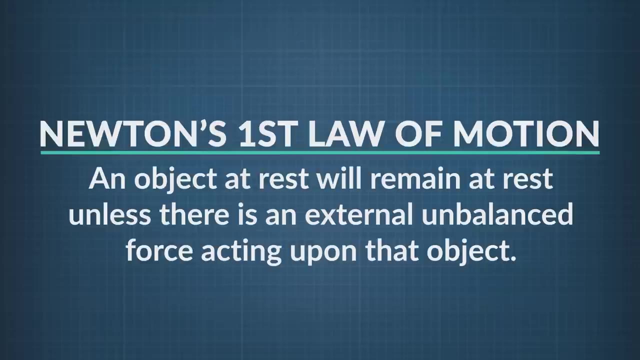 side than the other. The difference between the greater and weaker force is that the greater force is the net force, I win. Now that you know about balanced and unbalanced forces, let's speed right into Newton's first law of motion. It states: any object at rest will remain at rest unless there's an external. 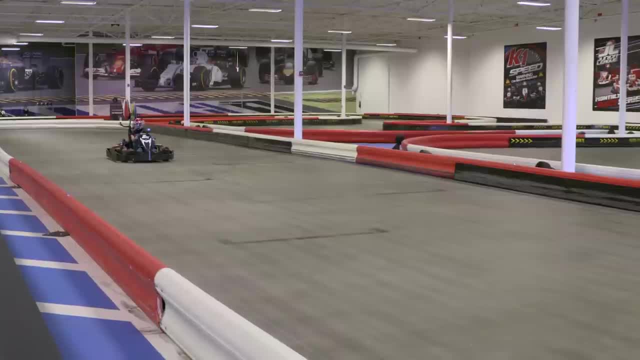 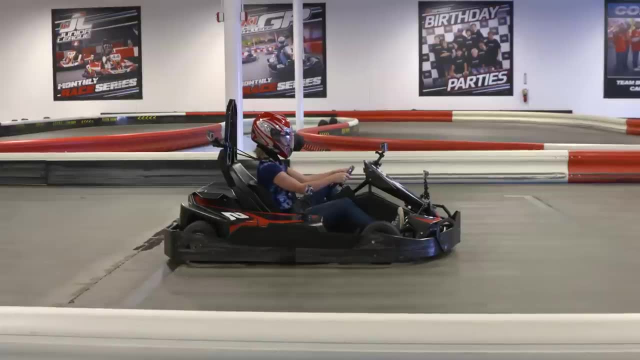 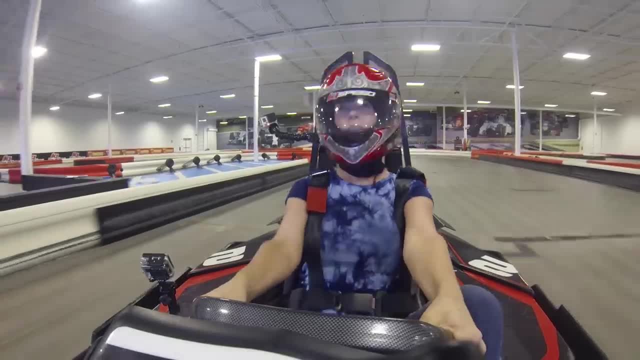 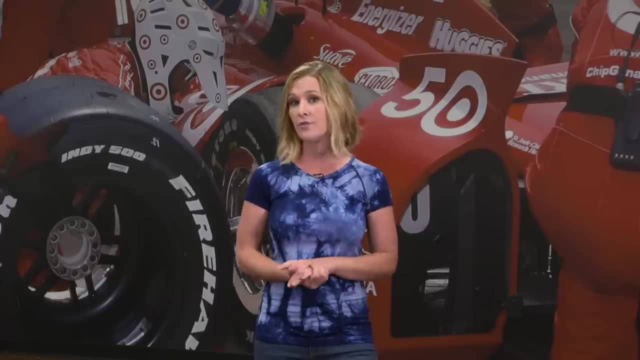 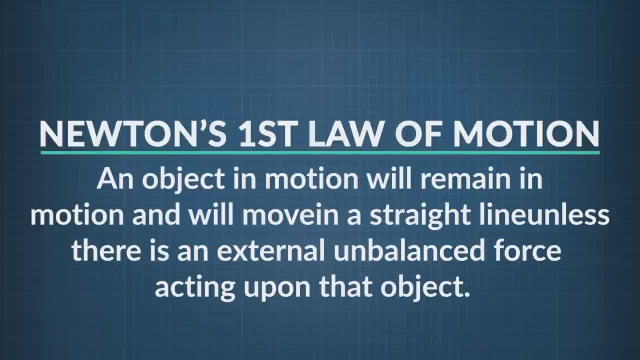 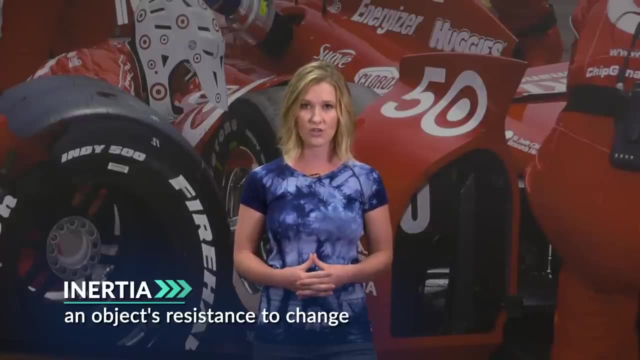 on to say that once an object is in motion, it will remain in motion and will move in a straight line, unless there is an external unbalanced force acting on that object. Newton calls this the law of inertia. Inertia is an object's resistance to change. So hit the 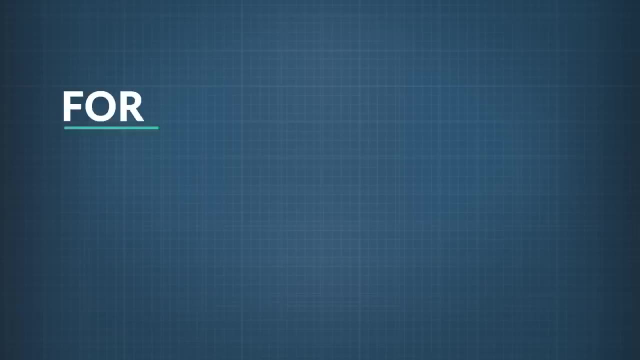 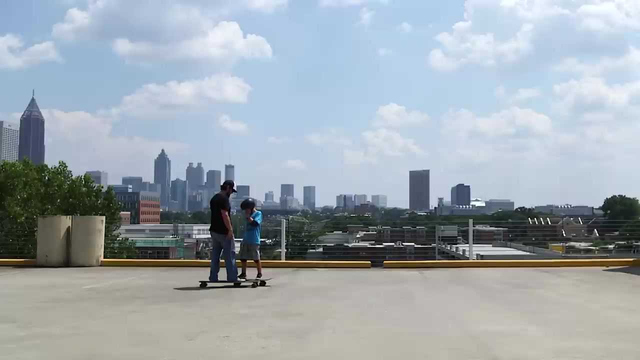 brakes and my body wants to keep going forward. And the more massive the object, the more inertia it has and the more resistance to change. Let's look at an example. What do you think will happen when a larger person and a smaller person push each other while 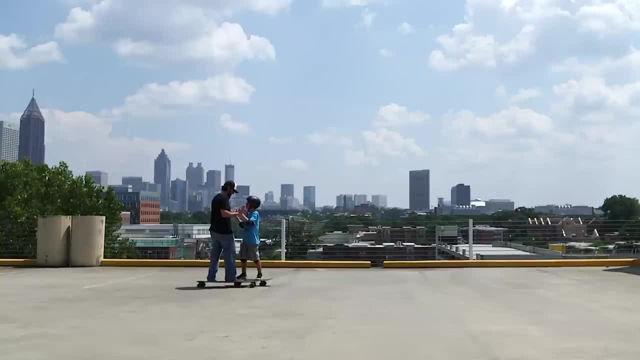 both are on skateboards. Who moves more? The larger person hardly moves, compared to the smaller person. Why is that? Because the larger person has more inertia. He's more resistant to moving. On the other hand, the smaller person is more resistant to moving. The larger. 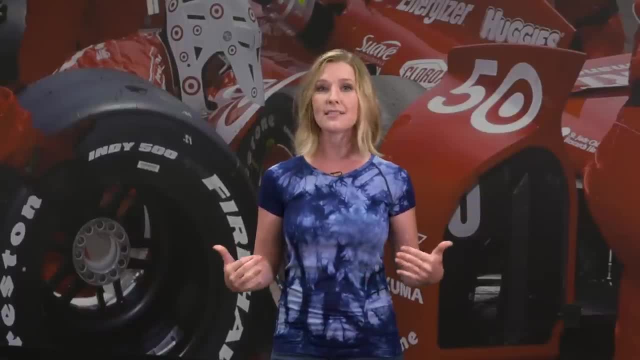 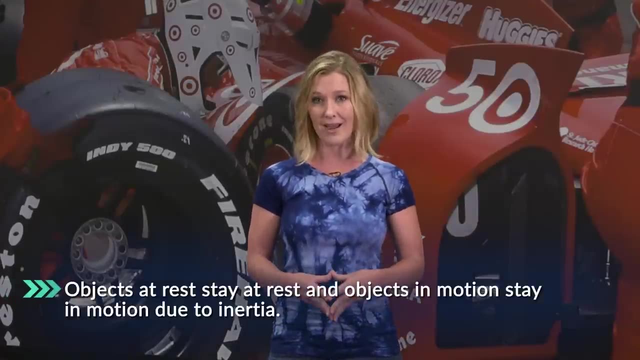 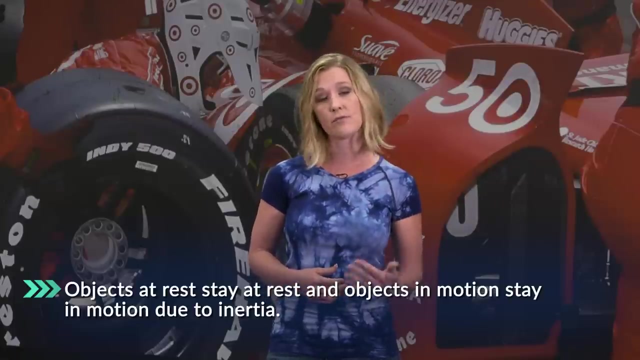 person is less likely to stay at rest because he has less inertia and is less resistant to change, so he moves more. So remember: objects at rest stay at rest, and objects in motion stay in motion because of inertia, which means they're resistant to the forces. 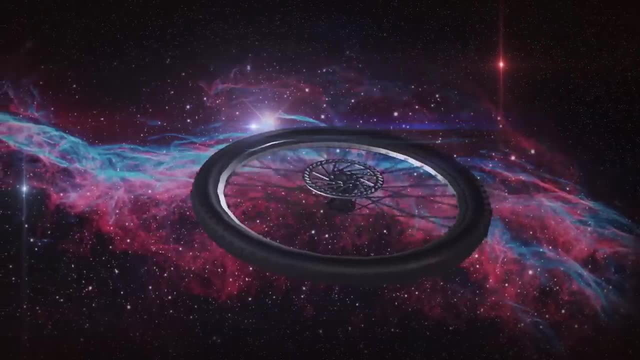 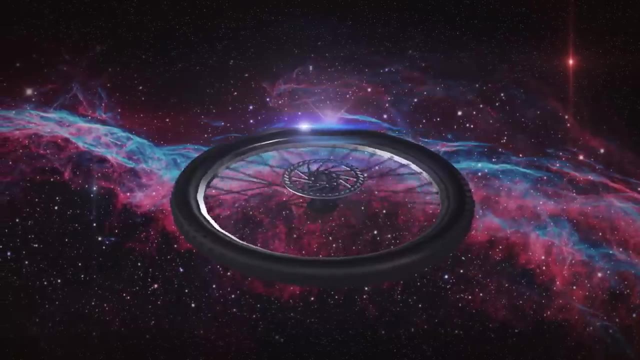 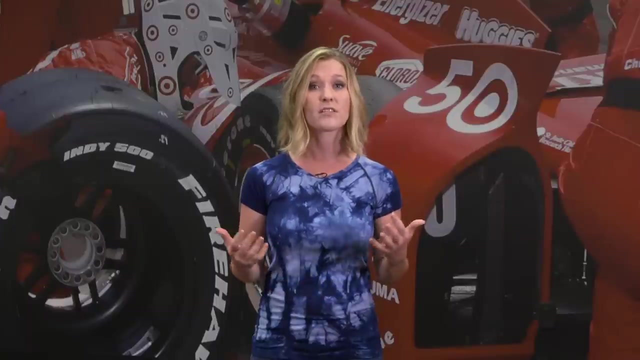 acting on them. Okay, so let's say you're in deep space and there are no forces like friction or gravity acting on an object like this bicycle wheel. How long do you think it will spin? It will spin forever at a constant velocity because of inertia and because there. 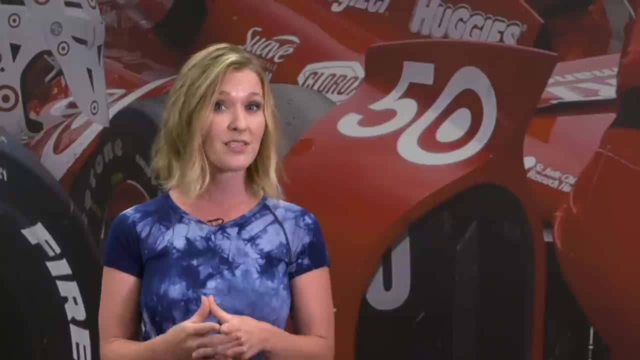 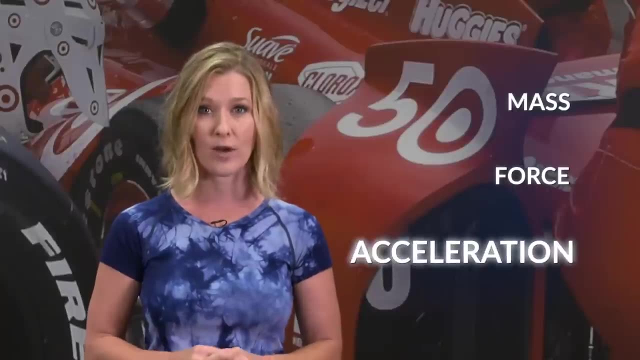 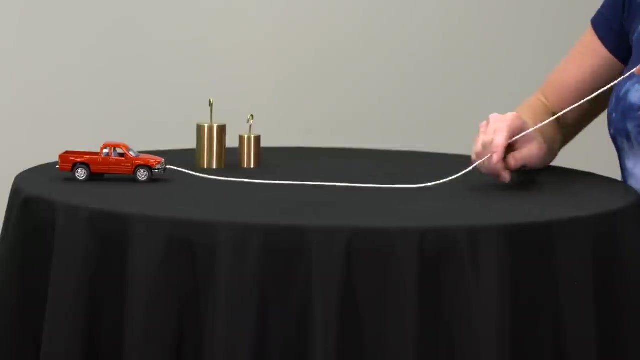 are no outside forces causing it to stop. Which brings us to Newton's second law. Remember these three words: mass force, acceleration. How do these three variables interact? Let's use this truck. If I pull the truck, it accelerates. If I pull the truck, with twice the amount. 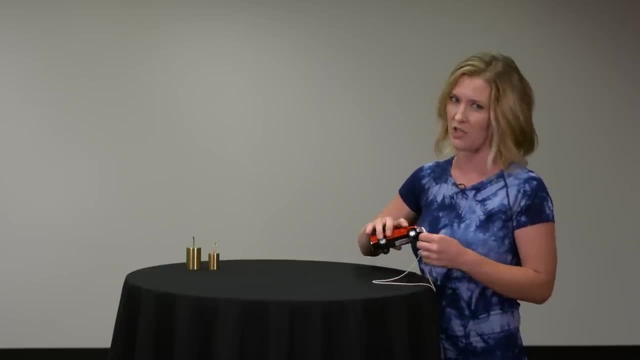 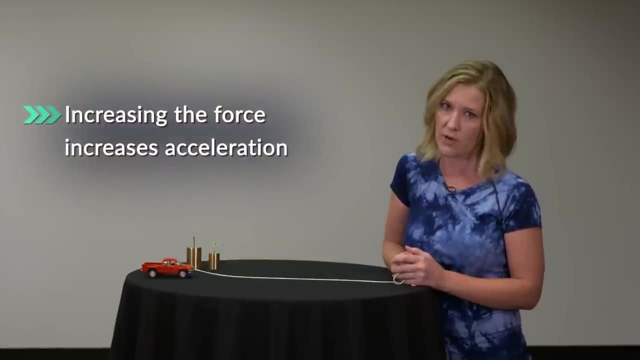 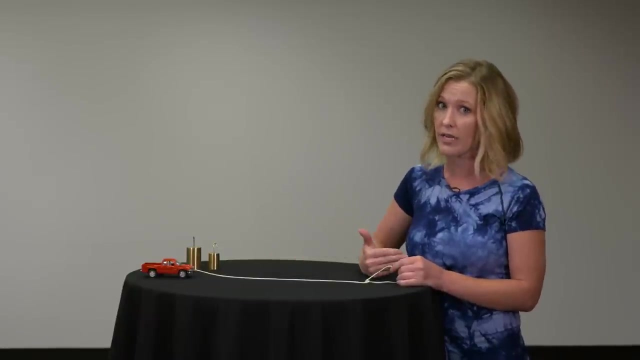 of force, it will accelerate Twice as much, Because force and acceleration are proportional to each other. if you increase the force, then you increase acceleration. The acceleration is always in the direction of the net force. The net force is moving the truck to the right, causing it to also 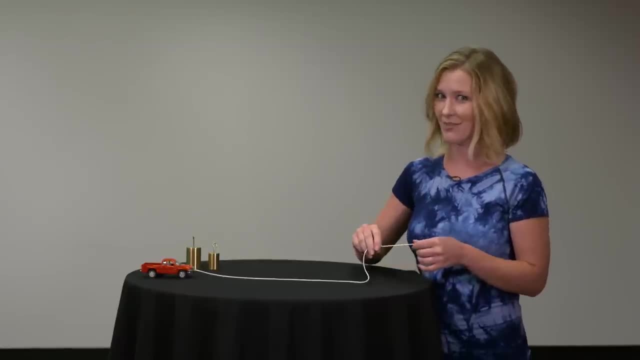 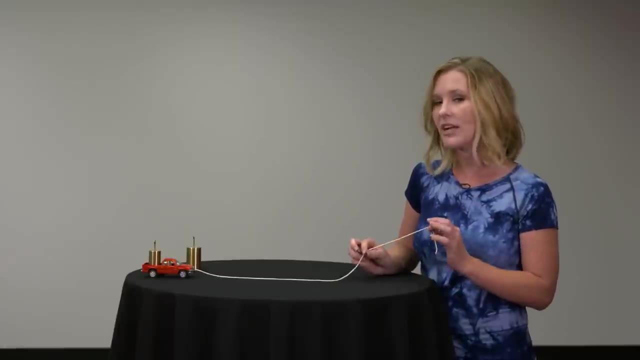 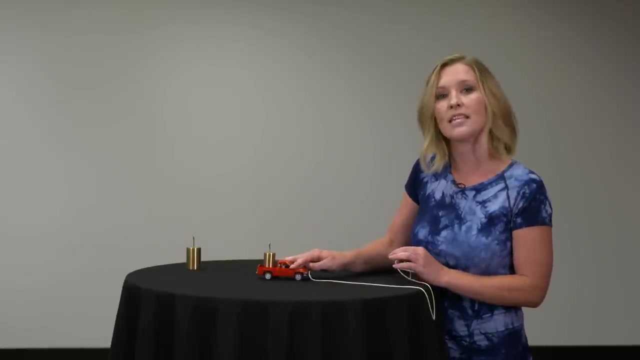 accelerate to the right. Okay, let's double the mass of the truck by adding this weight. How does that affect acceleration? When I double the weight of the truck and pull it with the same amount of force, it accelerates. What is the force? It will accelerate half as much Given the same amount of force. the 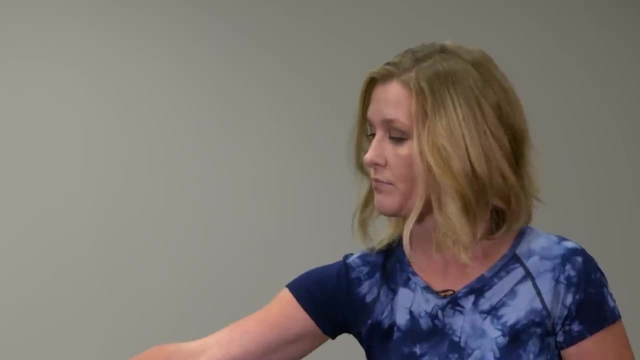 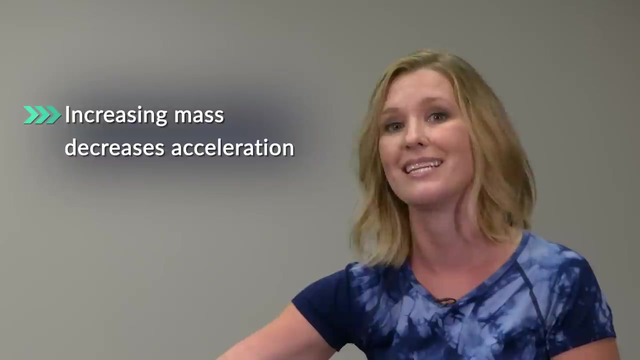 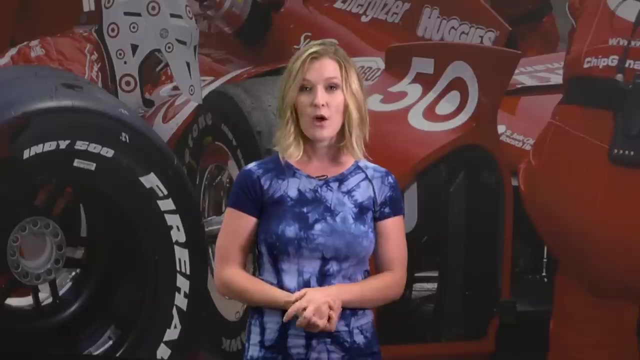 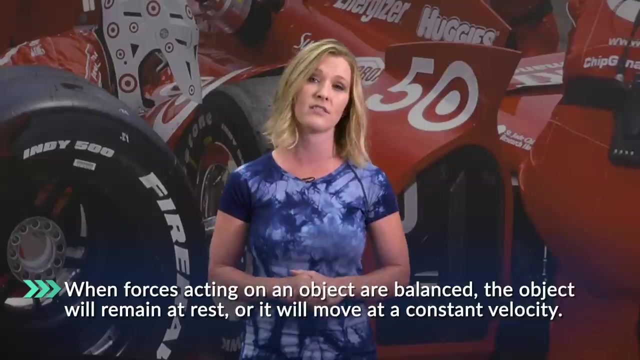 heavier truck accelerates slower. Now, mass and acceleration are inversely proportional. given the same amount of force, You increase the mass and decrease the acceleration when the force stays the same. Okay, here's something about forces you should know. When forces acting on an object are balanced, the object will remain at rest or it will move at a constant. 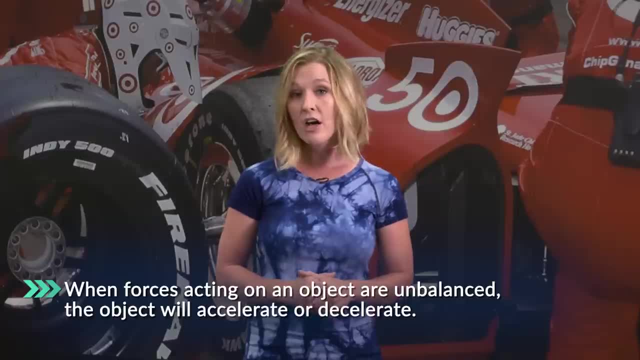 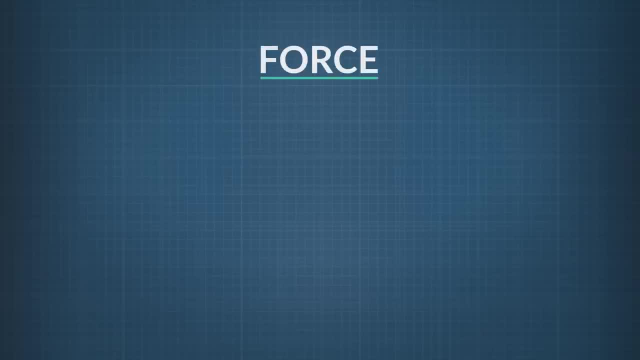 velocity. When forces acting on an object are unbalanced, the object will accelerate or decelerate. So when I hit the gas on the car, the force from the tires pushes on the track, causing an unbalanced force on the cart which causes the cart to accelerate. 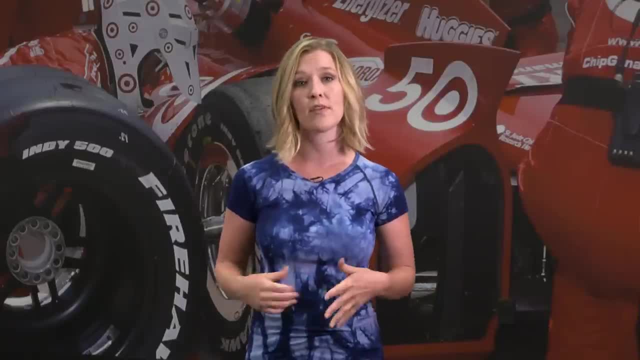 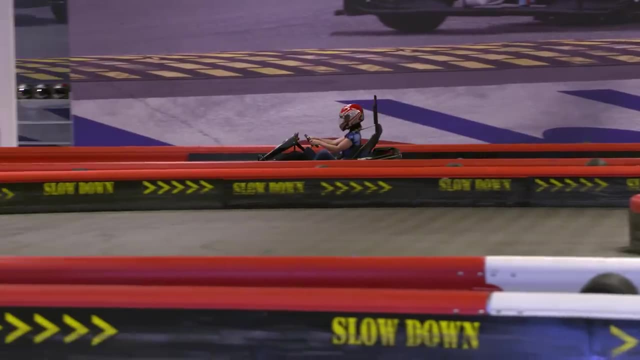 If the cart is already moving and I push on the gas just enough to move at a constant velocity, then all the forces on the cart are balanced. Forces that could slow the cart include things like air resistance, friction between the tires and the track.